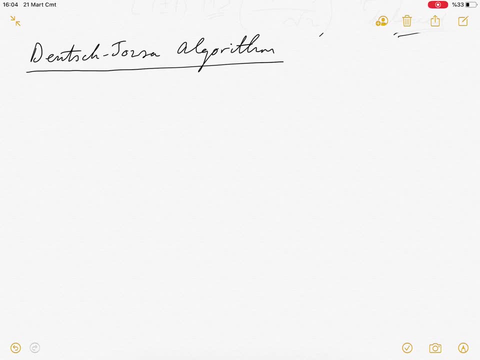 Okay, so in this video we will talk about a simple generalization of the Deutsch problem called the Deutsch-Jozza problem or the Deutsch-Jozza algorithm. Now, in the previous algorithm, the function was defined from a binary set- 0, 1, to 0, 1.. 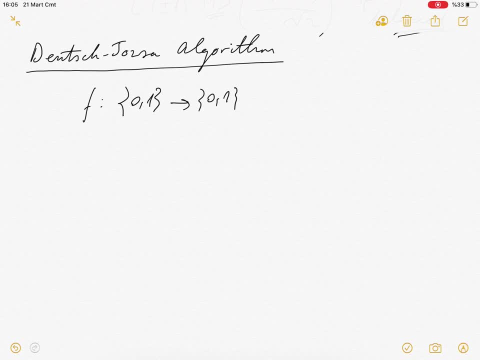 Now, in this case, in the Deutsch-Jozza problem, the given function is from 0, 1, to the n to 0, 1.. Okay, Alright, so now we assume that f is given as a black box, similarly as earlier, and we assume that f is either constant. 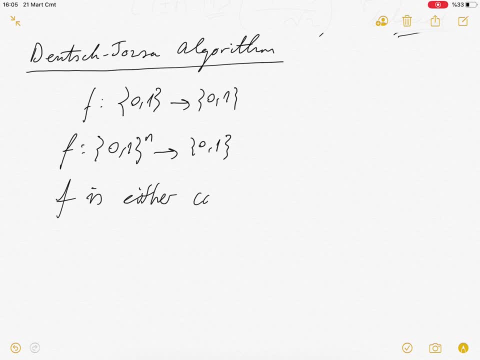 so assumption f is either constant, meaning that f of x is all the same, is all the same for all x in 0,, 1, to the n. Okay, So we assume that f is either f is either a constant function or a balanced function. 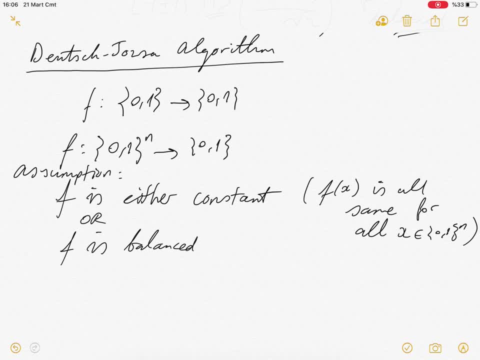 In this case, balance means that f of x is 0 for exactly half of the inputs and it's 1 for the other. So it's 1 for the other half. okay, so it's half half. For half of x, f of x is equal to 0, and for other half, f of x is equal to 1.. 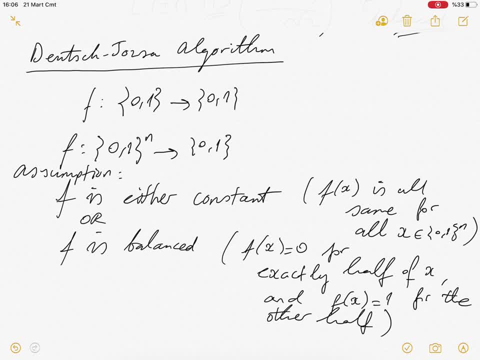 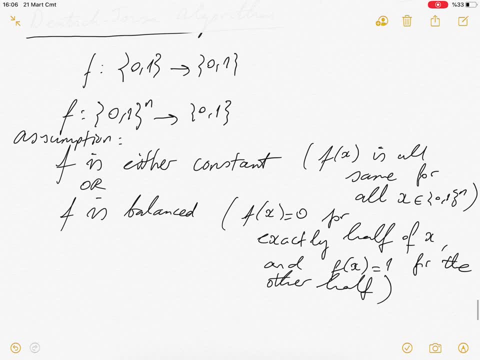 Okay, It's not some other ratio, it's not like 1 to 3 ratio, it's exactly half half. Okay, That's our assumption. So, for instance, if f was a function from 0, 1.. 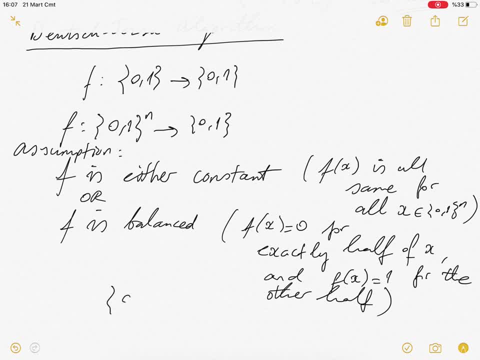 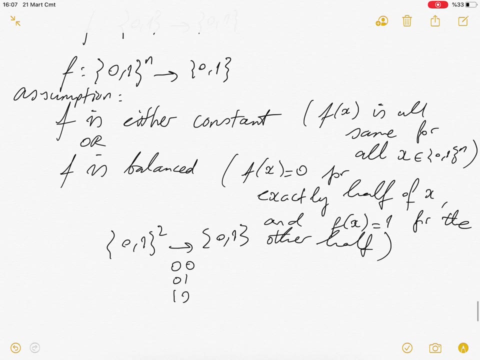 to 0, 1 over 2 to 0, 1,, then that means there are four cases right: 0, 0, 0, 1, 1, 0, 1, 1.. Function f is balanced if for exactly two inputs it maps to 0,. 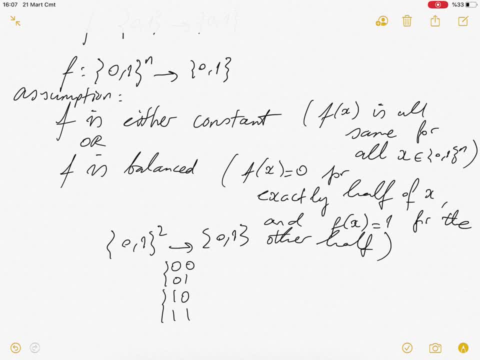 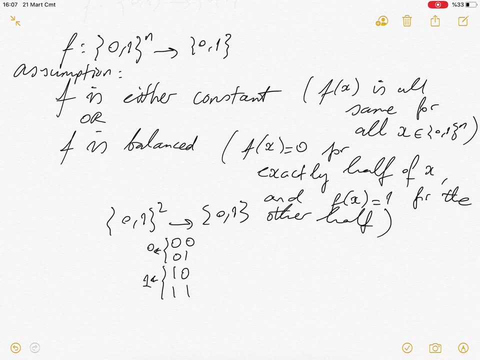 and for the other two inputs it maps to 1.. Okay, So it's exactly half half. All right Now, and the problem is the same. Given f as a black box, the quantum version of f, of course we're talking about uf. 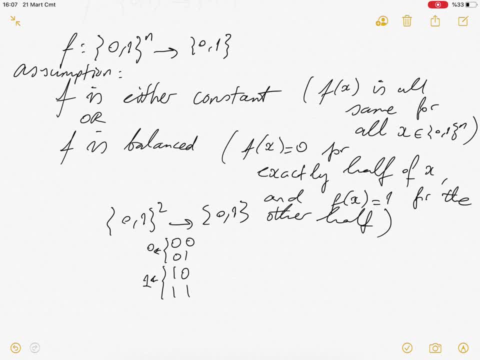 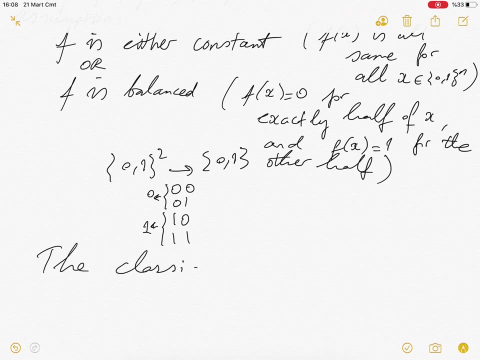 and we're going to define it in a moment. We want to know whether f is a constant function or a balanced function. Now, classically, using classical algorithms, the solution requires- at least the classical solution requires- how many queries? Well, it requires 2 to the n minus 1 plus 1 queries, right? 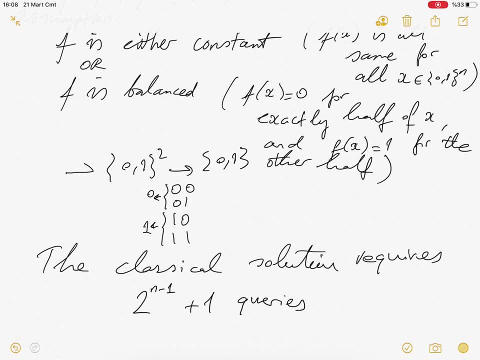 In the worst case. so let's think about this function. In the worst case, what we could do is that we could evaluate f for all inputs, right, And there are four cases here. so it's 2 to the n divided by 2.. 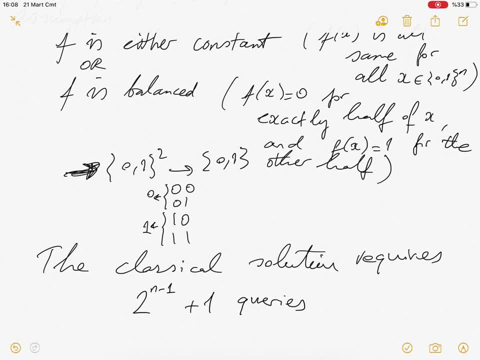 That's 2 to the n minus 1.. If it's all 0 up to this point, we need to evaluate one more right plus 1, to see whether the function is balanced or constant. If the next evaluation gives us 1,, then we know for certain that the rest of the outputs will be 1 as well. 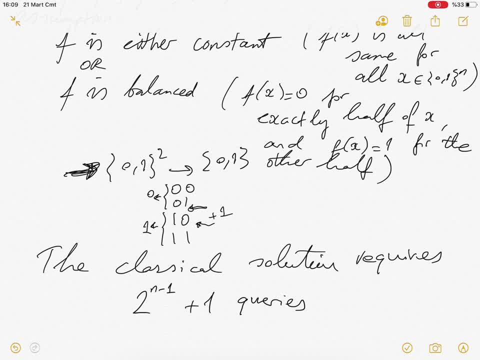 So we know instantly that the function is balanced in this case, but if it's 0, then we know that the rest of them will be 0 as well, And in that case we know that the function will be- will be- a constant function. 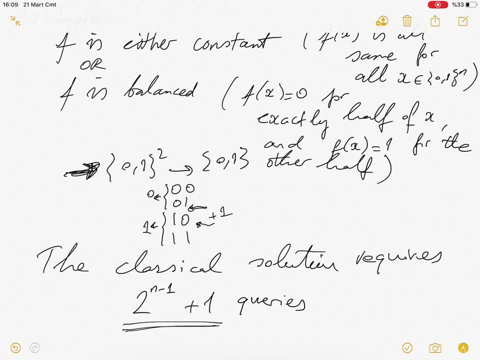 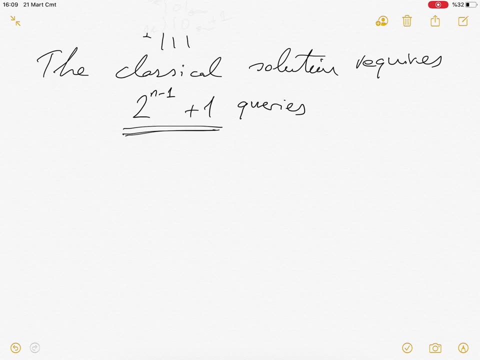 So it requires exactly this many queries to determine whether f is a constant function or a balanced function. Okay, now, surprisingly, using quantum computers and using an appropriate quantum algorithm, it only requires one query. Okay, It's only one, With only one evaluation of f. 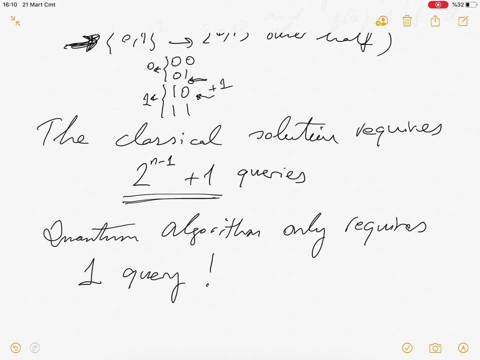 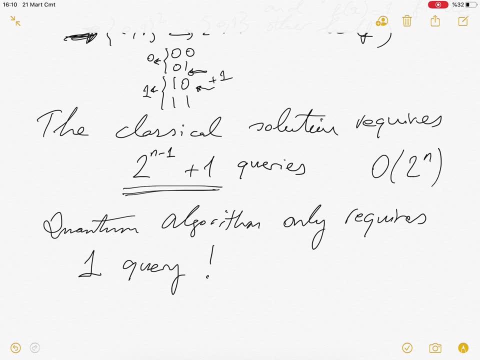 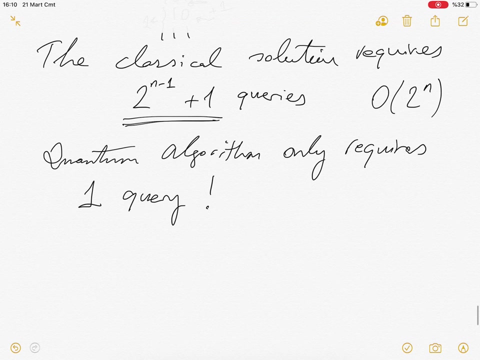 I can know whether that function, that given function, is constant or balanced. So we have an exponential speedup right. It requires exponentially many steps for the classical computer to determine whether a given function of this form is constant or balanced, whereas in 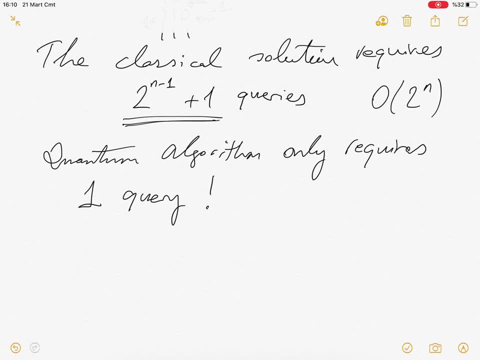 quantum computing. using quantum algorithm, it takes constant time. right, It's bigger than 1.. So let's see how to solve this problem. Now f is given as a black box. Of course we want the quantum version of f. 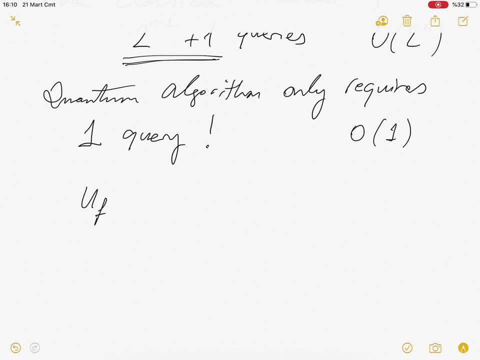 So uf will denote the quantum version of the function f and uf is a. uf will be given as a black box. Okay, that means we can evaluate uf but we cannot look inside and how it's defined inside actually. All right. 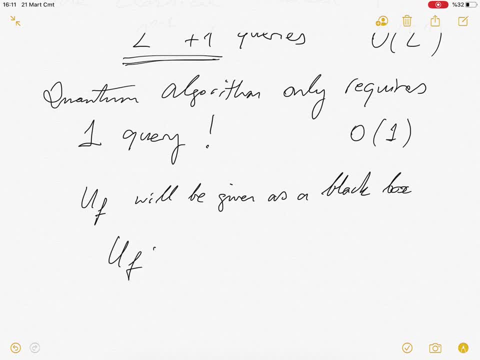 So uf, similarly, will be given in the form of, and the first register of uf will be an n-bit string. okay, an n-bit, an n-qubit register. And to separate this from a one-qubit register, I'm going to use a boldface. 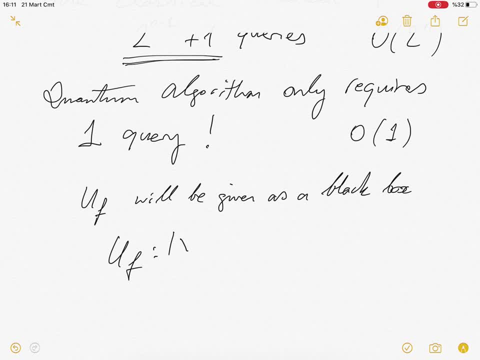 In the lecture note I use a boldface letter, So let me denote the boldface cat x, meaning that x is an n-qubit register. Okay, Boldface x. Okay, Okay, Okay, Okay, Okay, Okay Okay. 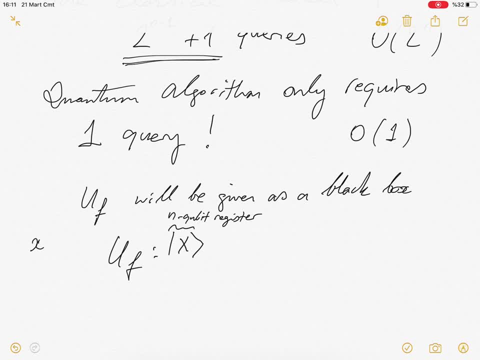 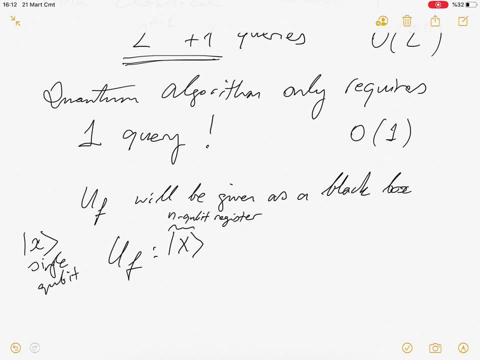 And then in the second input of uf, we have a one-qubit register. All right, Y, okay. and then this maps to X, remains the same. and then the second qubit maps to Y, X or F of bold X, alright. 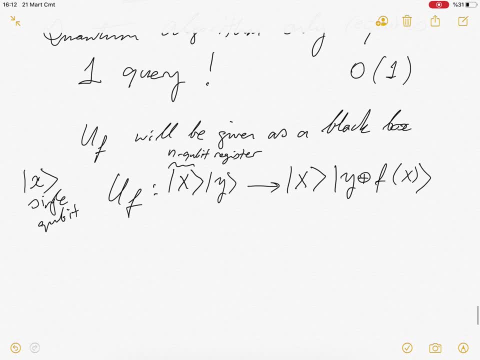 so U, F, X, U F. X, dependent on X, is controlled by the register of N qubits in state of bold. X, that is the N qubit register. okay, Y is the control qubit and X is the target qubit here. so again. 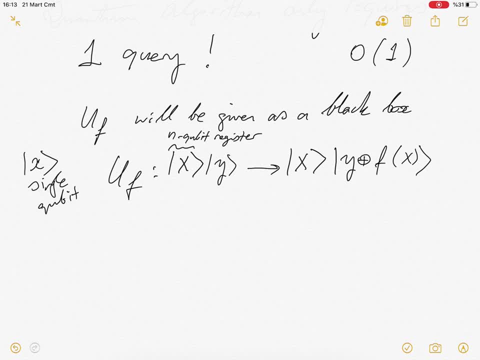 given such function, given such a unitary transformation U F, X, as earlier, the minus phase superposition state 0 minus 1 over square root 2 is an eigenvector of the function U F, with eigenvalue minus 1 to the power of F of bold X. 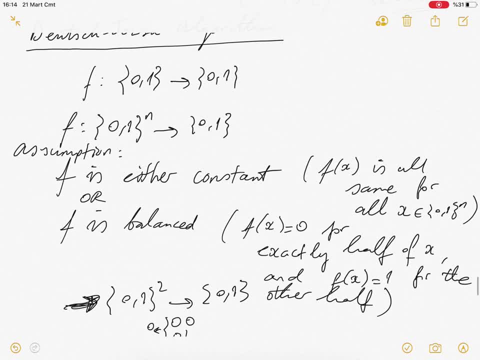 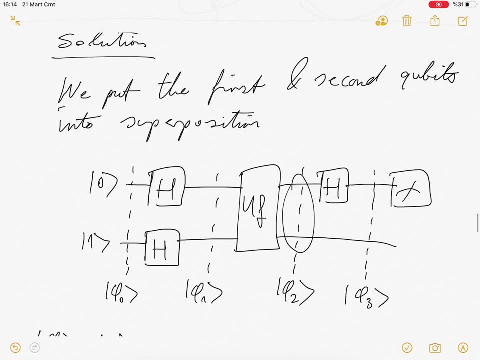 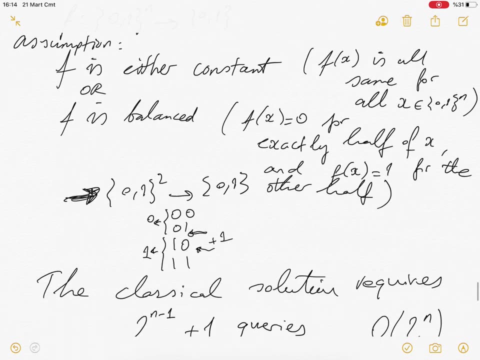 okay, we saw that earlier in the earlier problem, in the second attempt, right right here. okay, so let's keep that in mind. okay, so I'm going to give the okay. so I'm going to give the okay, so I'm going to give the. 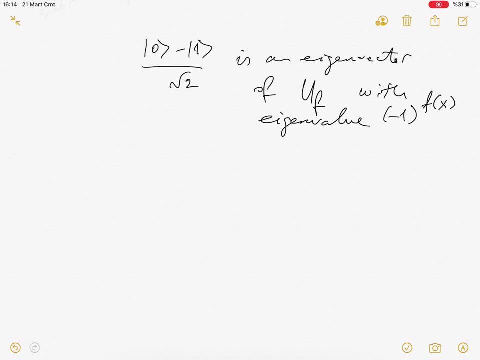 give you the solution straight away and without bothering with with wrong solutions. now let me draw the circuit diagram for the dot Joseph problem. it's actually given on page 65 in the lecture notes. okay, but let me draw it here and then explain step by step. so UF is given as a black box. UF has two inputs: the 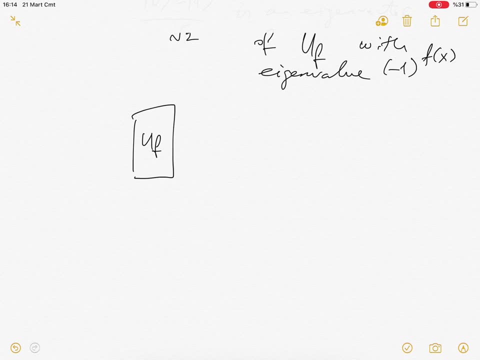 first input is an N qubit register. so we start with, we started, all zeros. let me make this bolt. okay, this is all. this is end qubits, all in zeros. okay, and I'm going to apply a Hadamard transform and N qubit Hadamard transform. 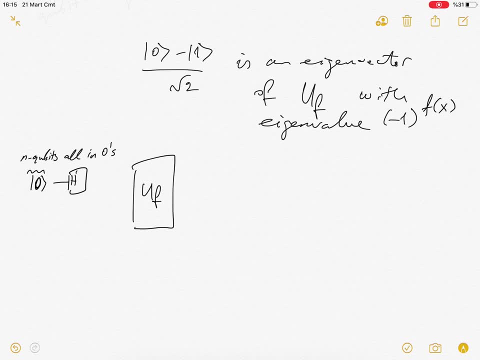 so H to the power tensor n. okay, this is an n-qubit Hadamard transform. this will go directly to as as the first qubit, the first inputs to UF and my control bits. I'm going to start with cat 1: apply a Hadamard transform. this will be our second input of UF and then in the outputs. 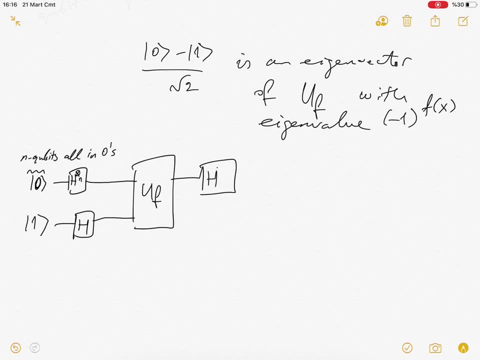 I'm going to apply another n-qubit Hadamard transform. okay, I'm not going to do anything with the second output and I'm just going to measure this n-qubit register. okay, so this is all and and qubits and qubits wires, whereas the second input is is just one qubits input. all right. 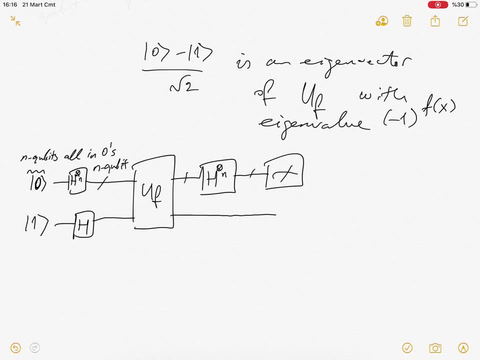 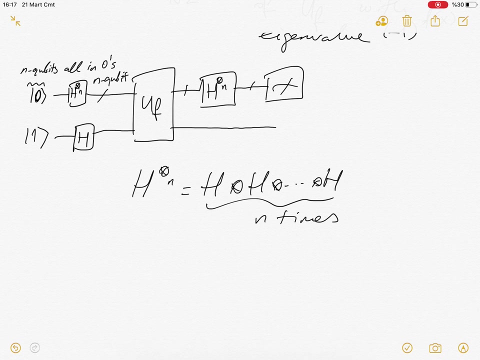 so H H tensor n is basically how the mark transform tensor Hadamard and many times, okay, this is how we define n-dimensional Hadamard transform. in the notes I also mentioned that this boldface 0 can also be denoted by 0 tensor n. okay, all right, so. 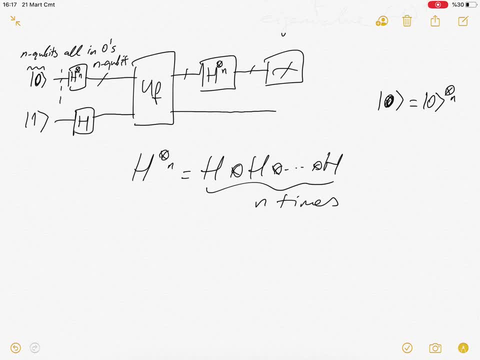 let's let's analyze the steps. suppose that this is psi 0, this is psi 1, this is psi 2 and this is psi 3. okay, so let's write each step then. all right, so the first step is to initialize the. so the first step is to initialize the. 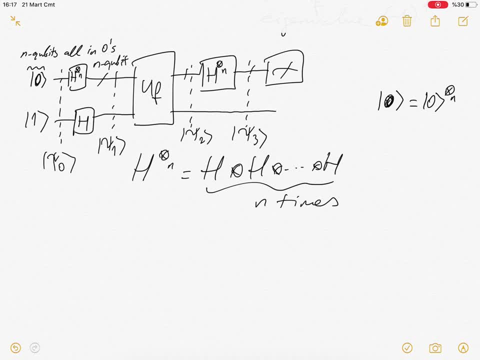 first input register to all zeros, okay. and then the second qubit is in state 1, so that means psi 0 will be in state 0. tensor n: tensor cat 1: okay, it's, it's an n plus 1 qubit input. okay, all right. now what happens if I apply a? 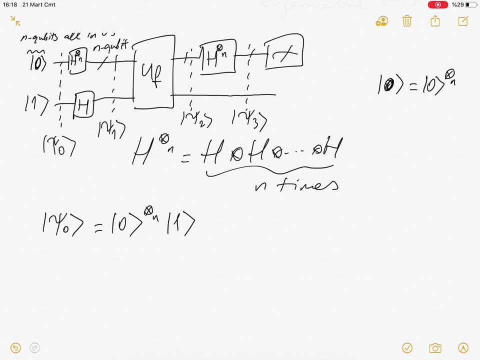 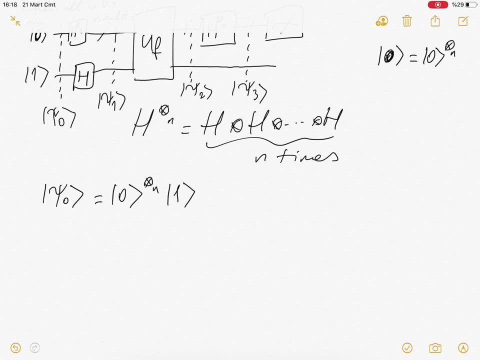 Hadamard transform and n-qubit Hadamard transform on an n-qubit register with all zeros. okay, now we already know the behavior of the Hadamard transform. a single qubit Hadamard transform on cat 0. it produces a superposition with the. 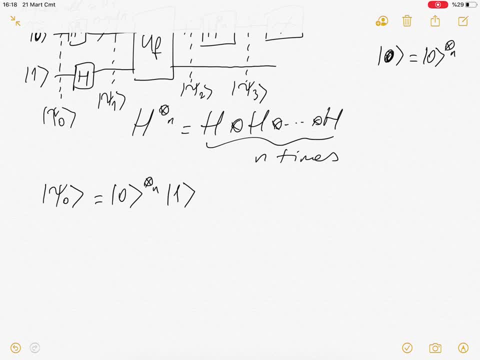 plus phase. but what about applying an n-qubit Hadamard transform on on an n-qubit register with all zeros? well, as you might expect, it's actually you're going to produce set of all strings of n-bit lengths with equal 1 over square root, 2 to the power n. 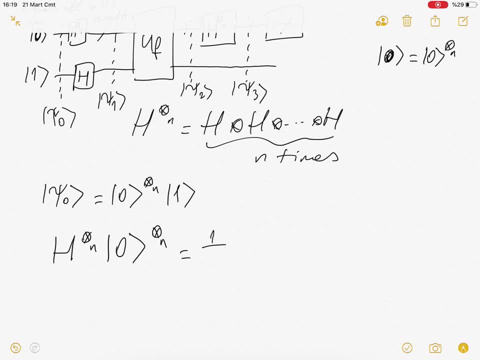 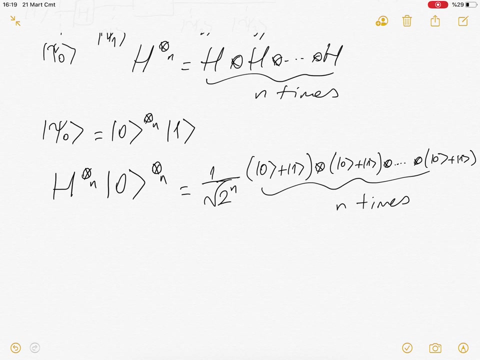 amplitudes. so it's going to produce all 0- 1 strings possible. now if you distribute these, you get all strings of zeros and 1's right, and this is n times like, So expanding this tensor product. if we write it more explicitly or if we formulate this so basically: Hadamard tensor n, applied on an n-qubit register with all zeros, will be basically equal to 1 over square root, 2 to the power n. 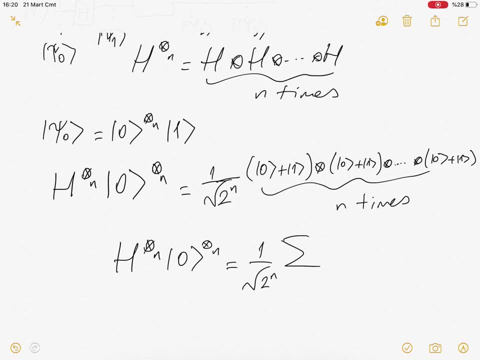 So summation: boldface x. and this is a string of n-bit length. cat, boldface x. So it's a summation of all n-bit strings with equal amplitudes. So the state Immediately after the first Hadamard transformation: psi 1, okay. 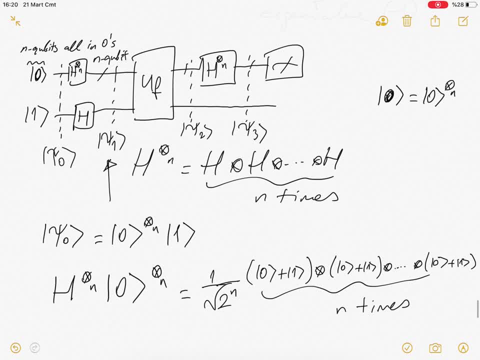 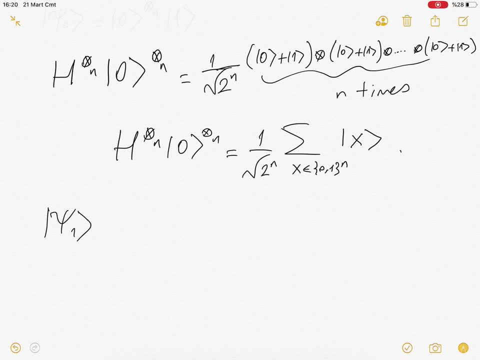 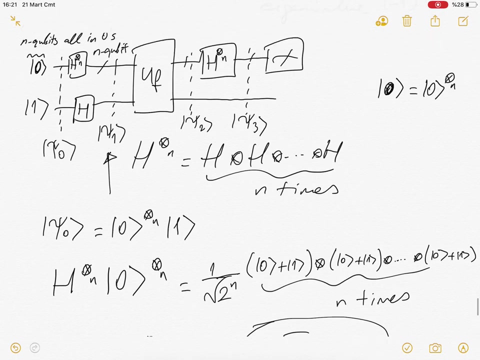 Now we're at this stage. Now we know the state of the first qubit, which is actually this superposition, But then we have also Hadamard 1 here, So the target qubit is in a superposition as well. 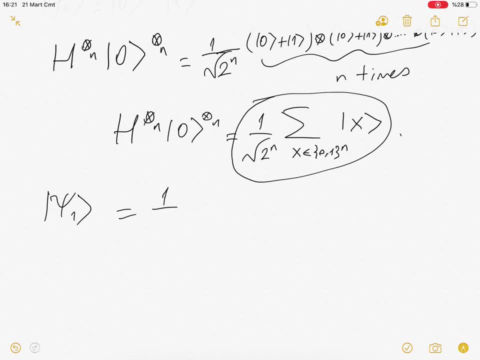 Okay, so psi 1 will be equal to 1 over square root 2, 2 to the n Summation X. So we get cat x And then we have 0 minus 1 square root 2.. 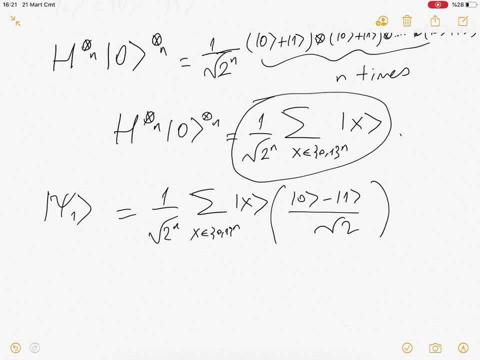 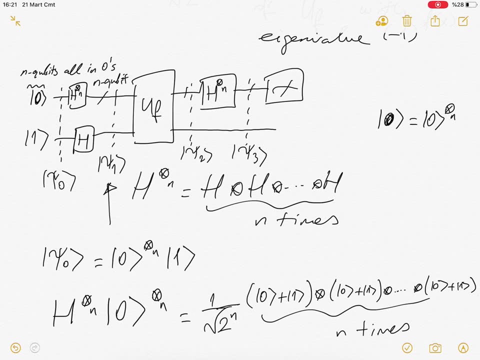 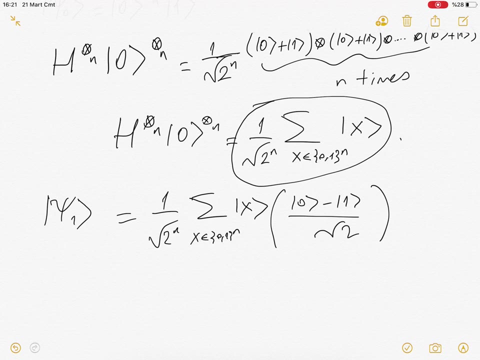 Okay Now, what happens if we apply UF here? Okay, Now let's try to write psi 2.. Remember that the target qubit is in a superposition, a minus phase superposition, So it's going to act as an eigenvector. 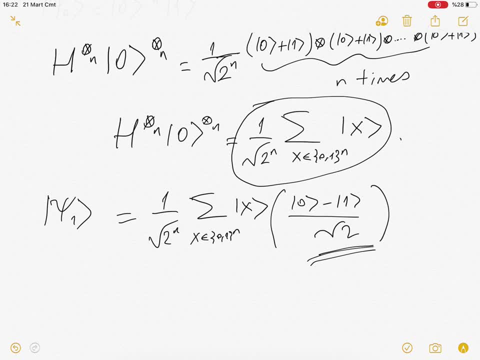 Okay, So because this superposition state is an eigenvector for UF with the eigenvalue minus 1.. So it's going to act as an eigenvector for UF with the eigenvalue minus 1 to the power f of x. 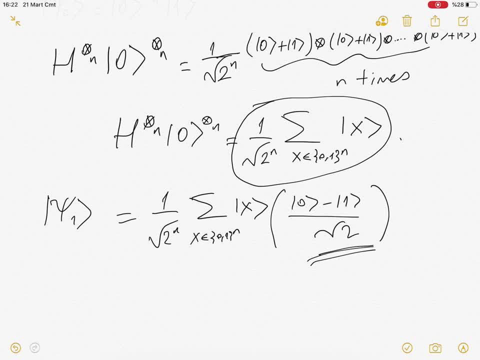 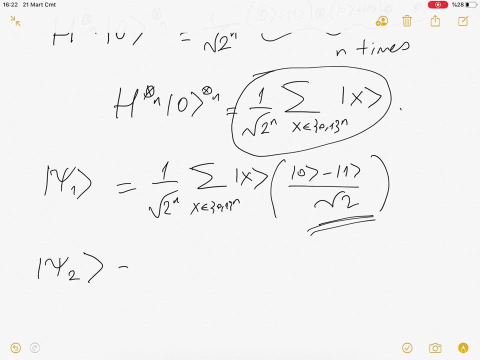 So we're going to have a phase kickback, okay, in front of the amplitude of the first qubit, the first register. So psi 2 can be written, as I'm going to apply UF on this whole state And it's going to be 1 over square root, 2 to the n. 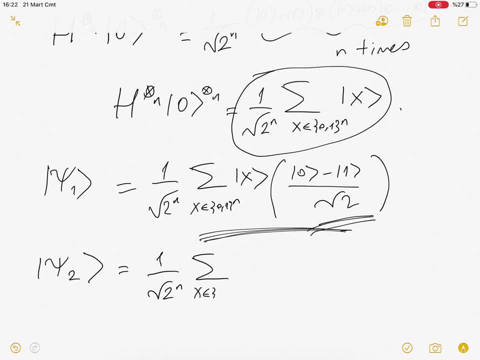 Summation: Summation Minus 1 to the power f of bold x. Okay, The first register will be the same x. The second register will be the same as well, because it's going to act as an eigenvector. 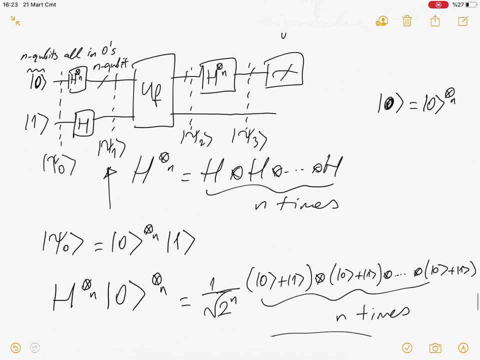 Right, So psi 2 will be. It's supposed to be this state. Okay, Now what happens if we apply the Hadamard transform on this bit? Okay, Because we're applying Hadamard transform on the first qubit and the first qubit is in a superposition of all n-bit strings. With amplitude of 1 over square root 2.. So we're going to have a phase kickback. So psi 2 is going to act as an eigenvector for UF, with the eigenvalue minus 1 to the power f of x. 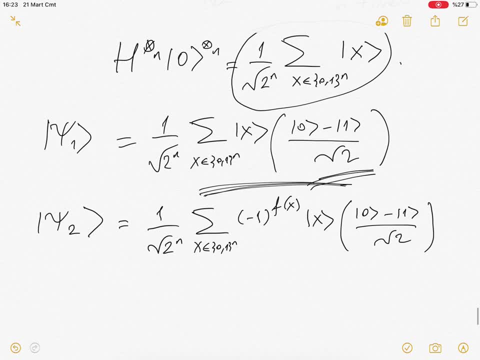 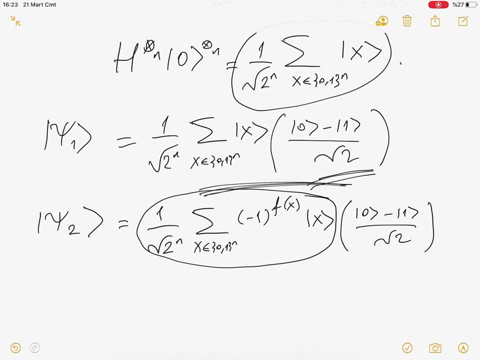 Summation, Summation, Summation, Summation, Summation of all n-bit strings with amplitude minus 1 to the power f of x. Okay, So let's look at how the Hadamard transform behaves on a single qubit input. 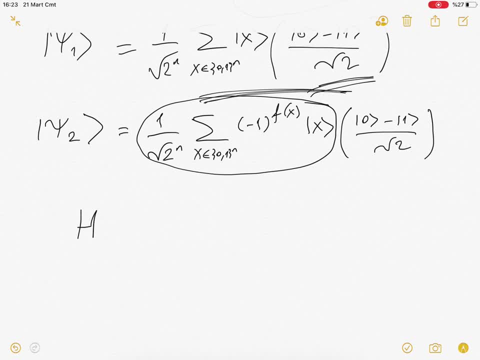 Okay, So I'm going to use this fancyx. It's a single qubit. Now we know that Hadamard 0 is basically 0 plus 1 divided by ket 2, and Hadamard 1 is 0 minus 1 divided by square root 2.. 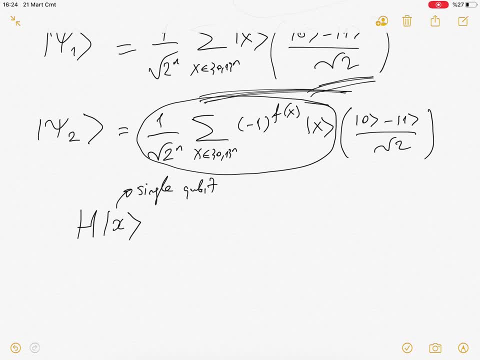 But generally speaking, if x is arbitrary, then we can formulate this as so: hx will be equal to 1 over square root 2, 0 plus minus 1 to the power x. So if x is 0, then this will be 0, right minus 1 to the power 0, it's 1.. 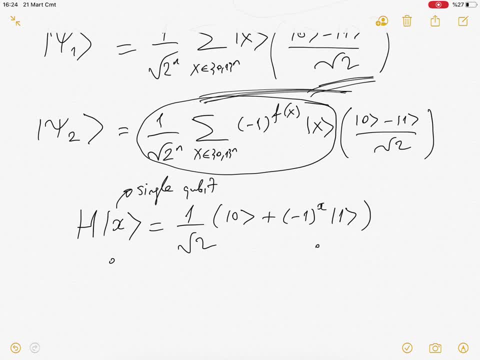 So we get, we get the desired outcome. it will be 0 plus 1.. But if x was 1, then we have minus 1 to the power 1. so we have, we have a minus phase in front of ket 1 and we still again get the desired behavior. 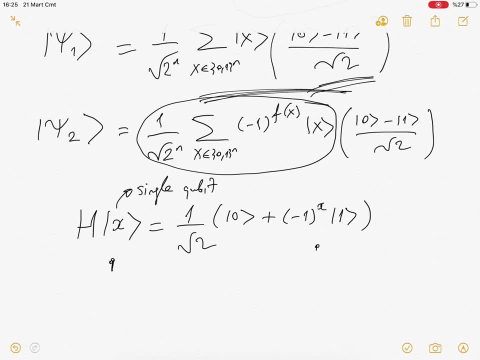 So it can be formulated in this form. but more generally this is equal to actually 1 over square root 2. we can write this in the summation form: z minus 1 to the power, x times z, ket z Right. What about the behavior of the Hadamard transform on an n-qubit register? 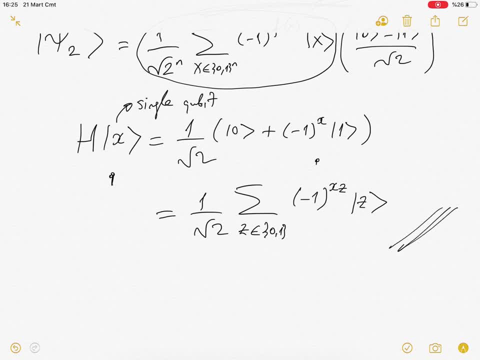 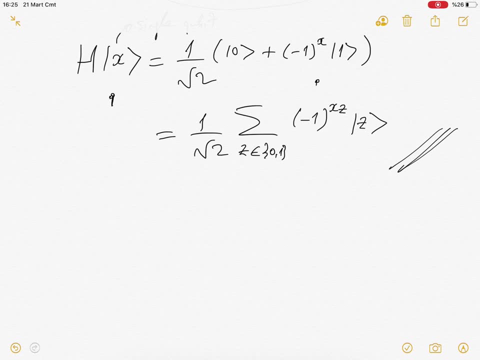 So let's keep this equation in mind And let's try to write the behavior of an n-qubit Hadamard transform on an n-qubit register. Okay, Okay, suppose that we have an n-qubit register, An n-qubit state, x, so this is can be written as: maybe x1 tensor, x2, xn. 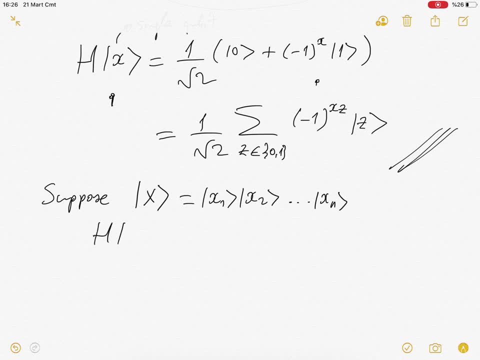 Okay, Now h of x is then h of x1 tensor, h of x2 tensor h of xn, And if we write this explicitly, this will be equal to 1 over square root, 2, 0 plus minus 1 to the power x1, 1.. 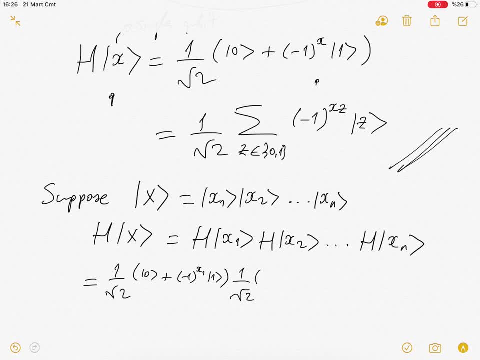 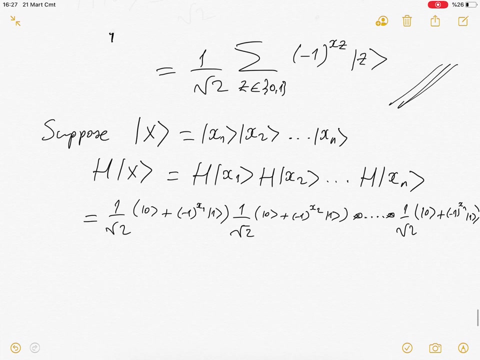 Tensor 1 over square root 2: 0 plus minus 1 to the power x2: 1.. Tensor Minus 1, sorry, 1 over 2 times ket: 0 plus minus 1 to the power xn 1.. Okay, now, using some algebra, I can rearrange this equation. using the summation formula, I can write this as: 1 over square root 2.. 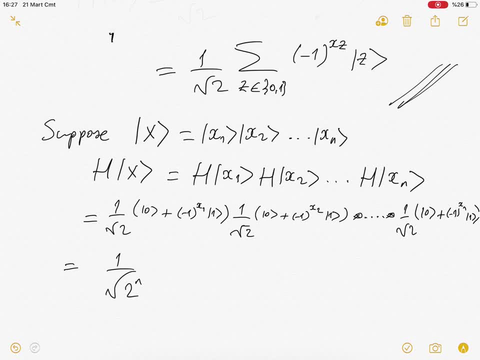 Over to the power n summation: z1, z2, zn. So this is an n-bit string. It's an element of 0, 1 to the n, So this will be equal to minus 1 to the power x1.. Z1 plus x2, z2 plus xn, zn. 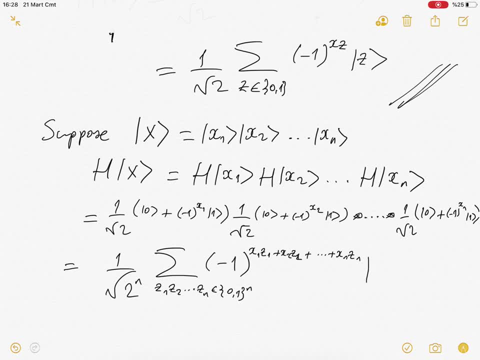 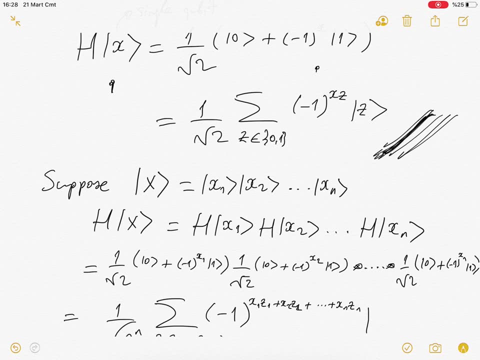 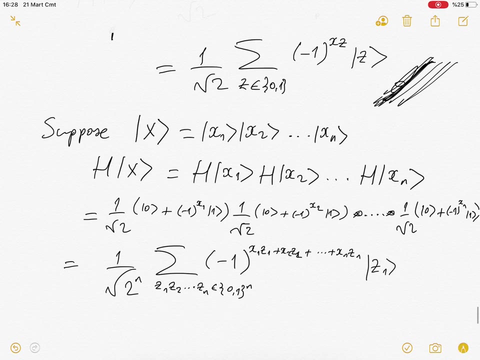 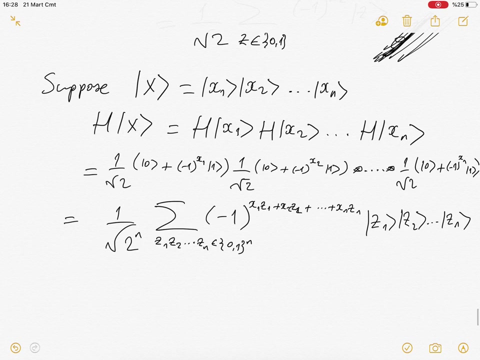 And then the state is: so I'm basically applying this formula. Okay, Right here. So this will be z1 tensor, z2 to zn Writing all together: h tensor n: n-qubit Hadamard transform applied on a n-qubit register on arbitrary state. 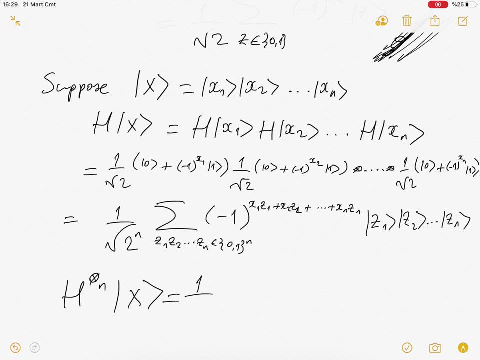 X is that can be written as 1 over square root. 2 to the power n. summation. boldface set. Okay, Okay, So that is an n-bit string Minus 1 to the power. boldface x times boldface z. 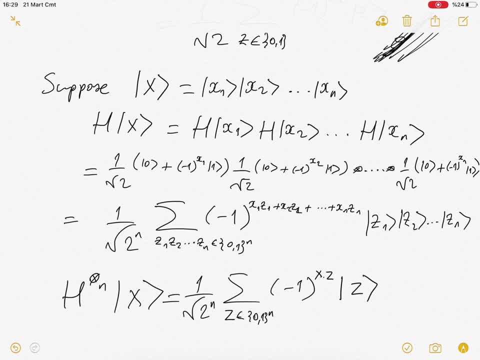 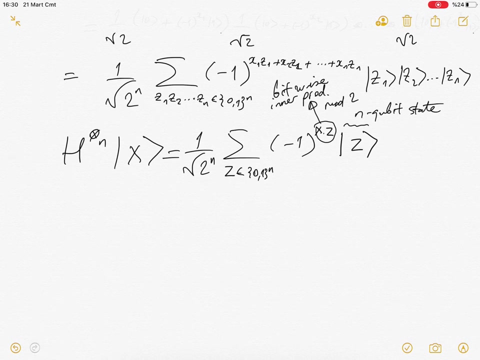 Ket boldface z. Okay, So this is n-qubit state And basically, x times z is the bitwise inner product of x and z modulo 2.. Okay, So this is bitwise inner product mod 2.. Okay, So let's keep this equation in mind, because we're going to use this often in the later algorithms. 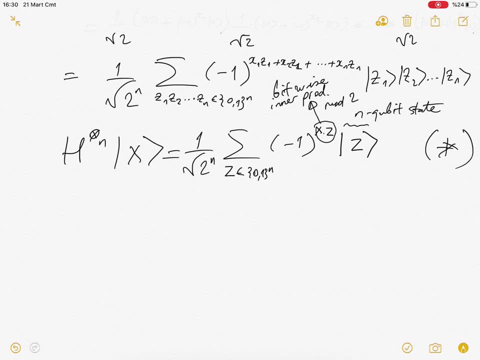 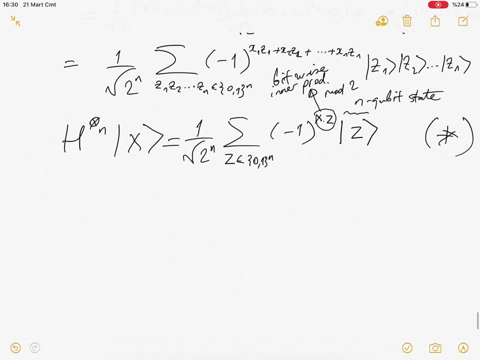 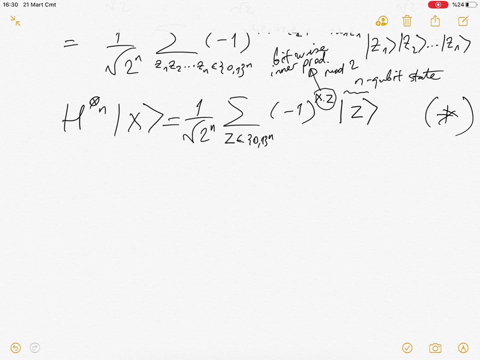 Okay, I'm going to put star here. Okay, So essentially, an n-qubit Hadamard transform on an arbitrary n-qubit register x in that way. Okay, So then psi 3, that is the state after the final n-qubit Hadamard transformation will be. 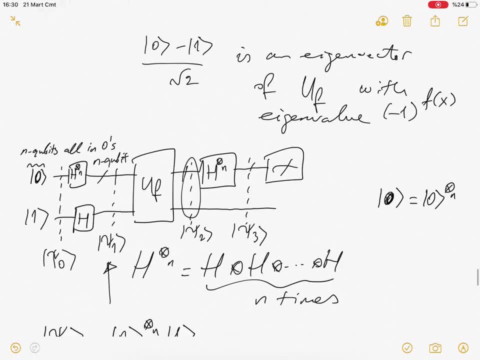 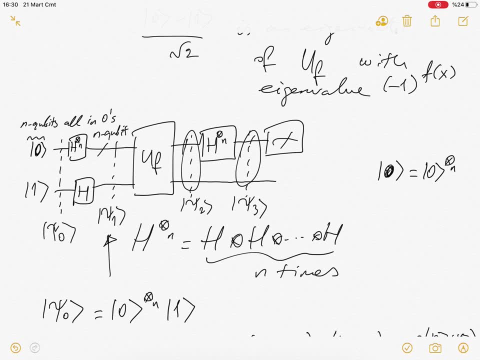 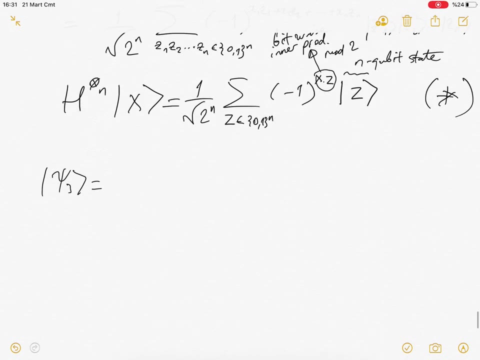 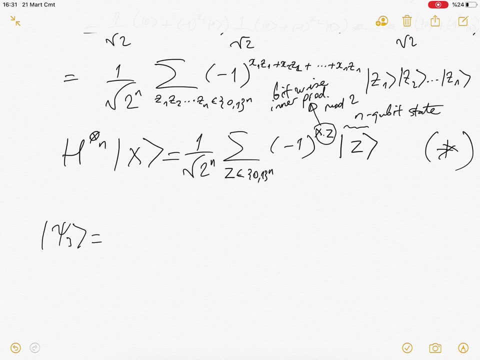 So psi 3 will be: Yes, we're here. Okay, We're going to write psi 3 after the n-qubit Hadamard transformation is applied on the first register. Okay, Okay, All right. So psi 3 then will be 1 over square root, 2 to the power n. 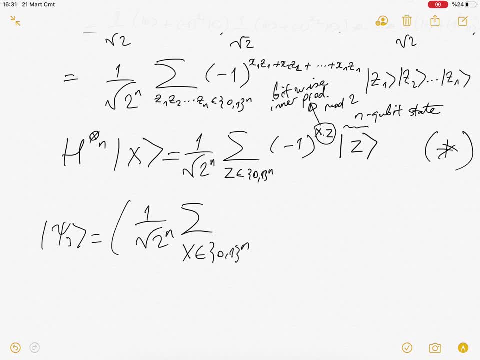 Boldface x And minus 1 to the power f of boldface x. okay, and then we have, and then we have this factor, I'm going to write this: 1 over square root, 2 n to the power n summation boldface set, which is an: 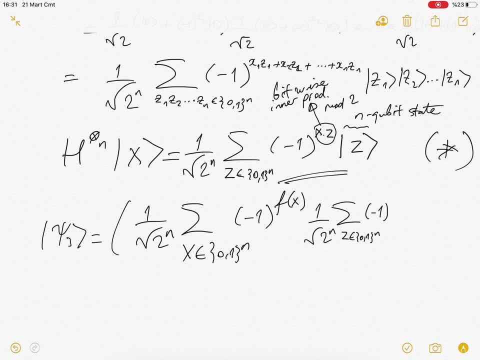 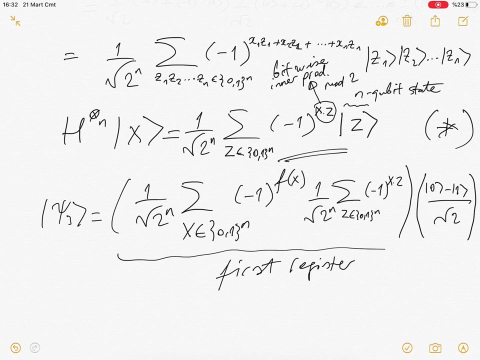 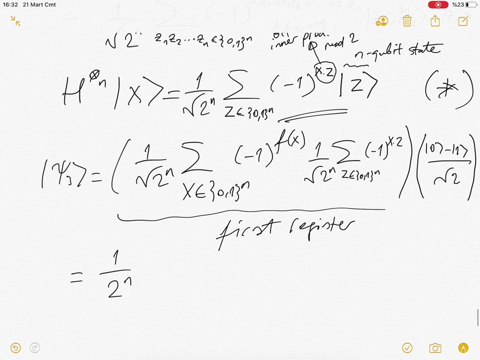 element of 0, 1 to the n minus 1, X times that. so this whole thing is our first register, okay, and the second register we have the minus phase superposition: 0 minus 1 divided by square root 2. okay, so we add the common factors, just rearranging the algebra we have, so I'll 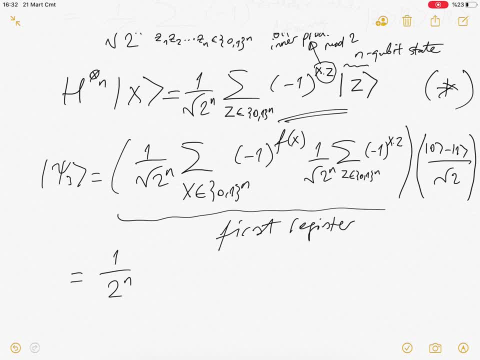 multiply the amplitudes, it will be 1 over 2 to the n. summation: boldface set 0, 1 to the n and then we add the common factors. so we add the common factors, we have the other summation: X 0, 1 to the n. the common factor is minus 1 to the. 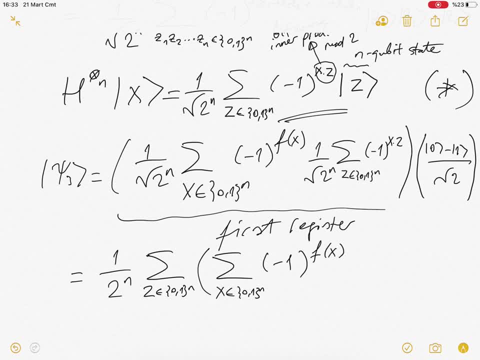 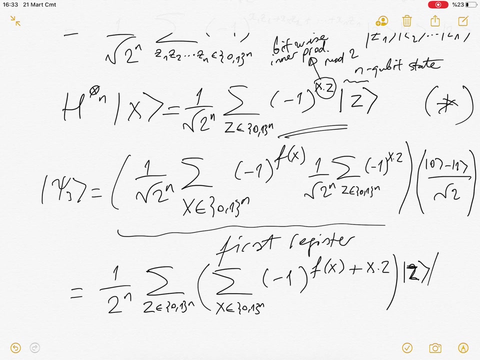 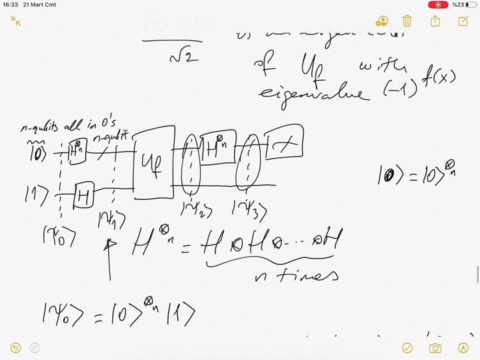 power F of boldface X plus. I'm adding the exponents X times boldface sets: okay, ZET is our first register. okay, and then the second register. I have the same superposition. okay, so psi 3 will be our final state here. okay, now we're planning to measure. 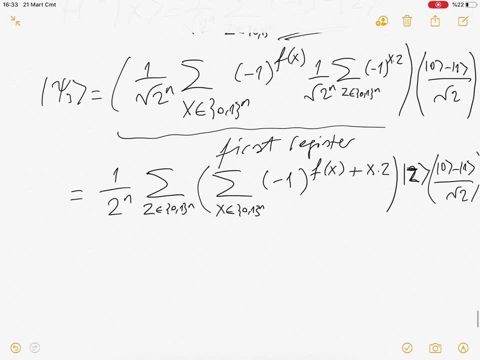 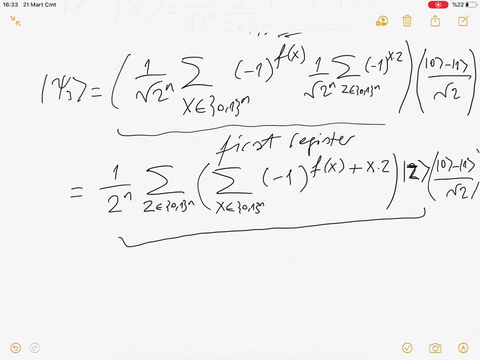 the first register and see what happens. okay, this will be our first register and this is actually. this part is our amplitude. although it looks a bit complicated, we will see in a moment that it's actually not, because we're going to take a look at one instance. so z here actually quantifies over the set of all zero one strings of n-bit length. 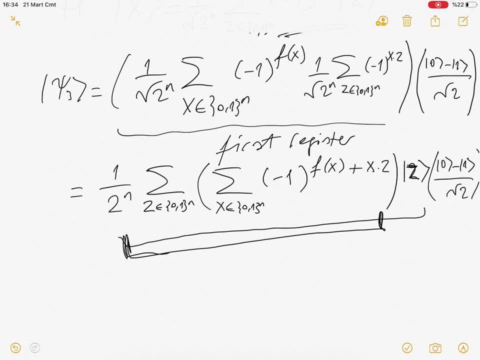 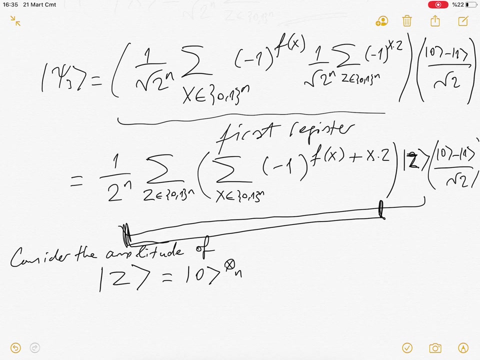 okay, but let's consider- so this is actually a superposition of all n-bit strings. but let's consider the components. when z is all zeros, okay, so let's let's consider the amplitude of all zero states. okay, now for all the when. when z is all zeros, this will be zero, right? so the amplitude of all zero state. 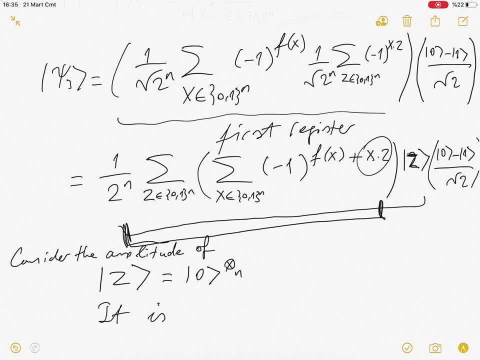 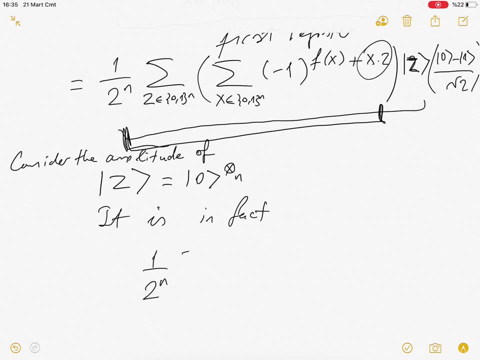 will be zero. it is in fact one over two to the n right summation, boldface x. it's minus one to the power f of boldface x. okay, okay, so this is the amplitude of all zero states, and then we will consider the zero, zero zero state, all zero states. 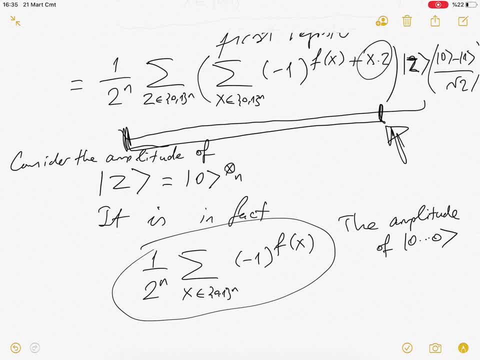 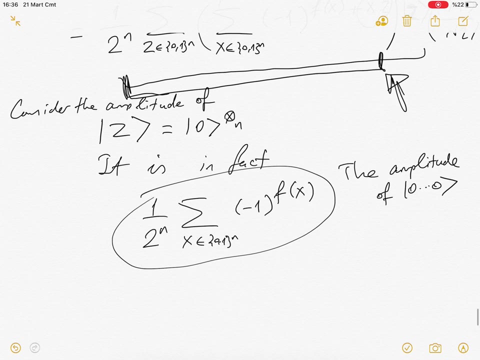 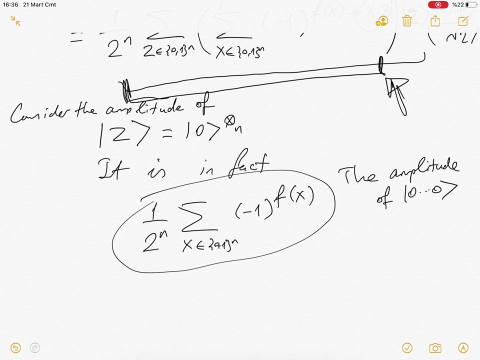 okay, in this superposition up here, we also have other uh or other combinations okay, with possibly different amplitudes, but let's consider the amplitude of all zeros now. So, depending on the characteristic of the function, whether f is constant or balanced, the amplitude of all zeros actually show a distinct, a unique characterization. It gets a unique value. 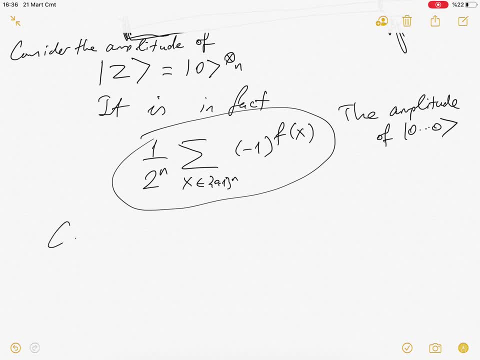 So I'm going to discuss the cases. Case one is if f is constant. Now let's consider what happens if f is constant, If f is a constant function, either for all f of x, f of x is zero or for all f of x. f of x is one. 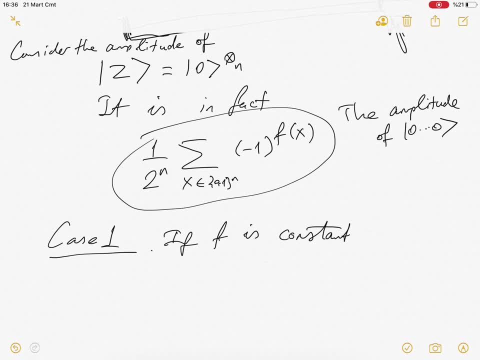 Okay, And depending on that, the amplitude of all zeros actually show a distinct, a unique characterization. So if f is constant, the amplitude of all zero states will be either one that is, plus one or minus one. okay, depending on the value of fx. okay, 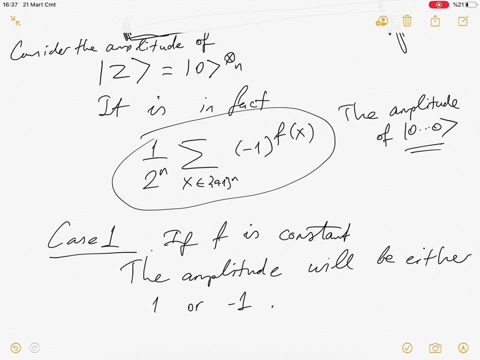 So if we measure, if we measure the first register, and if f is constant, if f is constant, well, the amplitude of zero, zero, zero state will be one. So it's going to return me, with hundred probability, the outcome of the first register, the outcome of the measurement, will be all zeros. 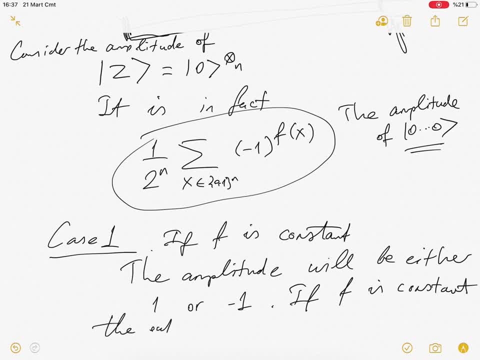 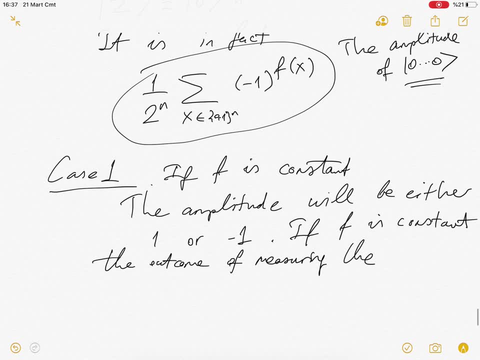 If f is constant, the outcome of measuring the first register- it will be one- Is, with probability, one is all zero states. So I'm going to observe all zeros in the first register when I measure it if f is a constant function. 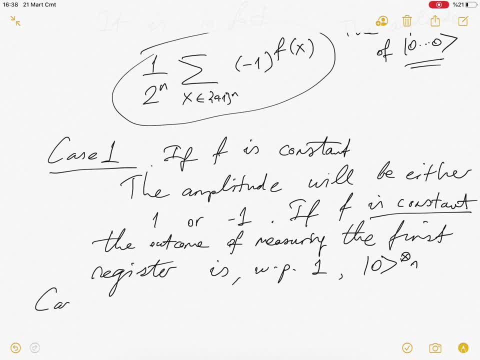 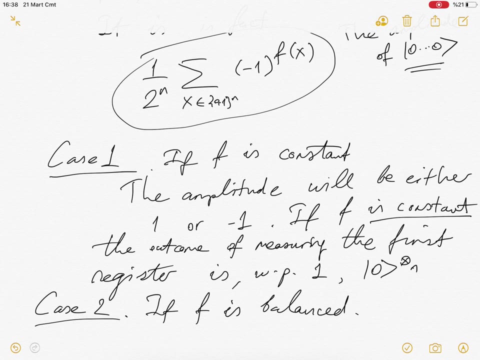 Alright. So what about if f is case two, If f is balanced? Now, if f is balanced, half of the f of x will be mapped to 0 and the other half will be mapped to 1.. But then if we look at the exponent, when f of x maps to 0, the amplitude will be equal. 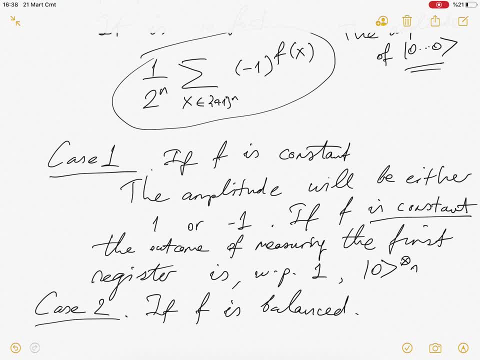 to 1, plus 1.. But if f of x maps to 1,, then the amplitude factor will be minus 1.. So for the first half, for one half, the total amplitude will be 1, and for the other half. 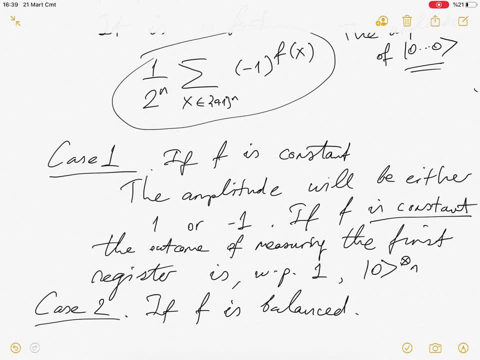 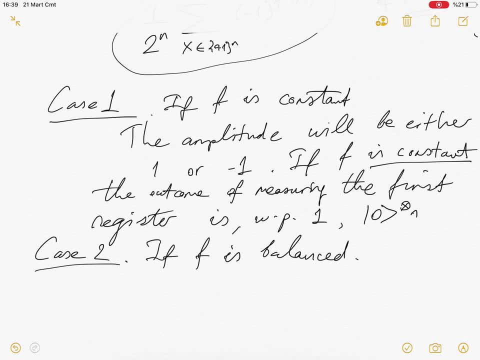 it will be minus 1.. And then the summation of all together will be just 0, right, So the positive amplitudes and the negative amplitudes, actually they intersect, They interfere with each other, so they cancel each other. 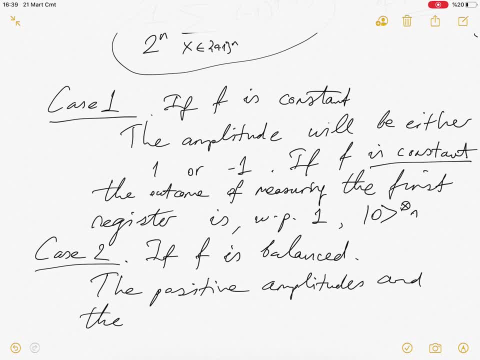 Half of the amplitudes will be positive and the other half will be negative and they cancel each other. So the total amplitude of this state- all-zero state- will be just 0.. So, upon the measurement of the first register, if f is a balanced function, it's impossible. 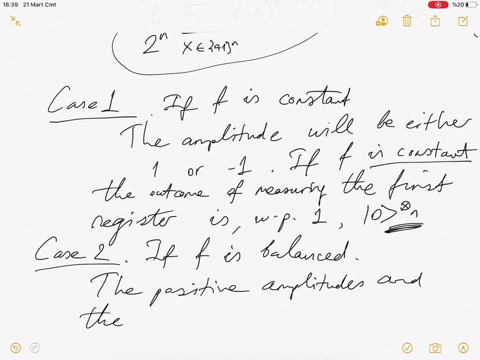 to obtain the all-zero state. I will not obtain. I will not see as the outcome of the measurement of the first register the state with all zeros. If f is a constant function, I'm certain that the first register, the measurement of the 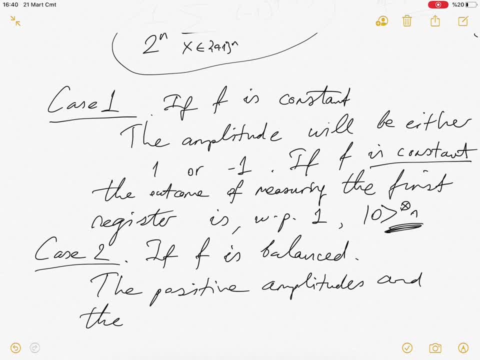 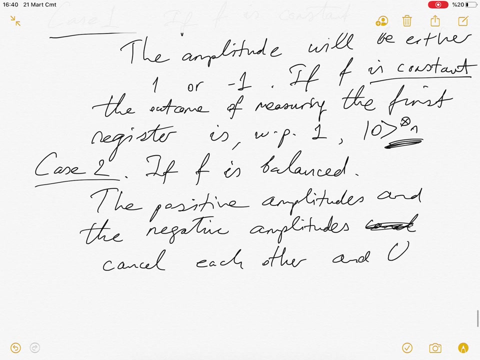 first register will return all zeros. Otherwise, if f is balanced with probability 1, it's impossible to obtain the all-zero state. So it's certain not to return all zeros. okay, So the positive amplitudes and the negative amplitudes cancel each other. 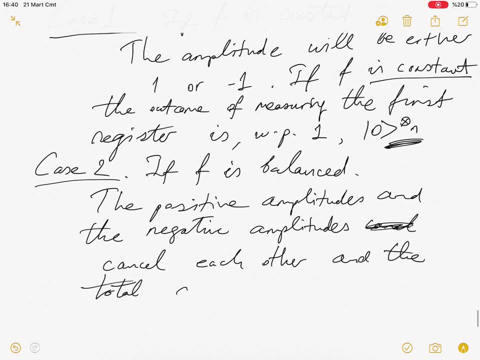 And the total amplitude. F is a constant function of f and f is a non-zero state. So if f is a constant function of f, f is a non-zero state, And if f is a constant function of f, f is a non-zero state. 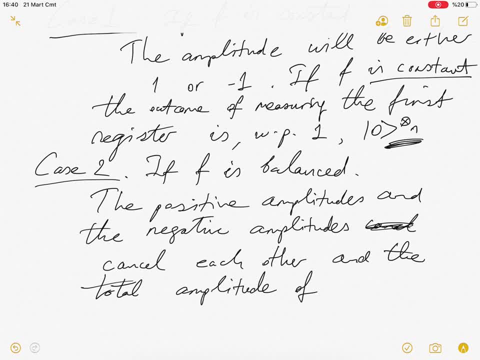 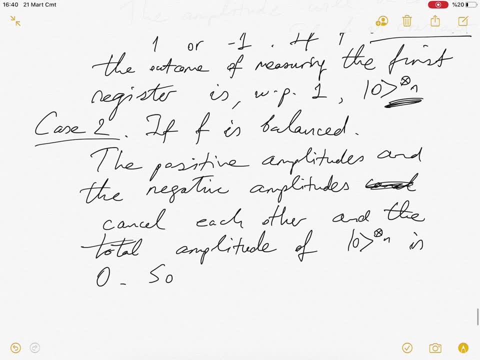 So if f is not a non-zero state, then f is a non-zero state of the state. all zeros is basically zero. so for certain the outcome will not be all zeros. so that means if I measures anything else but all zeros in the first register, then 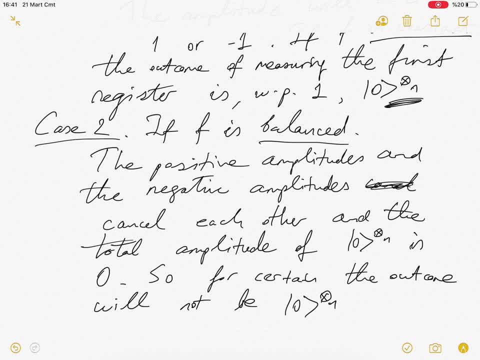 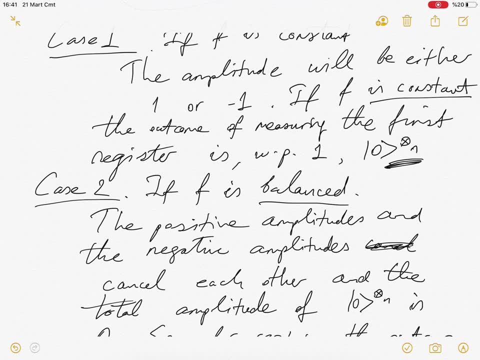 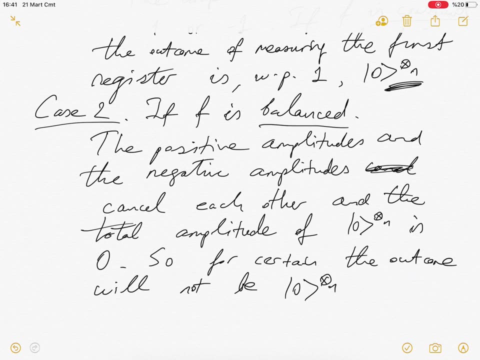 I know for certain that the function is balanced, but if I observe all zeros and I know for certain that the function is constant, okay, so this is how we have this dichotomy and how we can determine if a function is balanced or constant: by using just a single query and you can see the power of the. 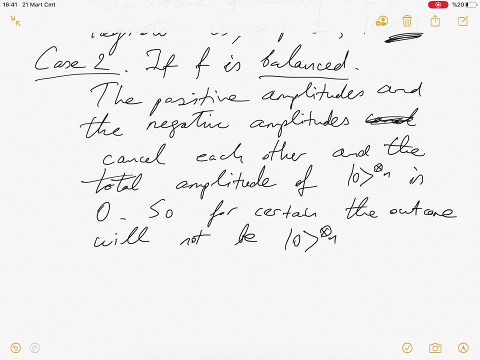 quantum algorithm over the classical one. whereas in the classical algorithm we need exponentially many queries, it's in the order of big O, 2 to the n, but in the quantum algorithm it's a. we have an exponential speed up, so it's we just use a single query. all right, so I'll see you in the next lecture. you.